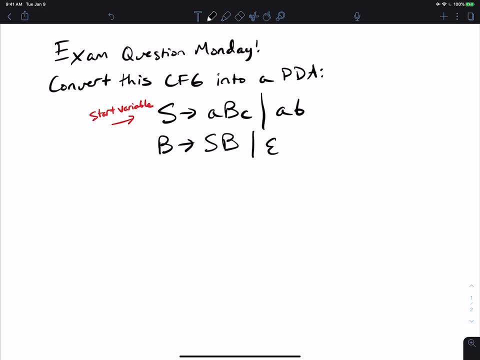 All right, welcome back to Exam Question Monday. Today we're going to be looking at this problem, which is very interesting in that there's a very simple procedure to do it, and a lot of students ask me about how to actually do this, So let's go into this. So we have a CFG given right here. 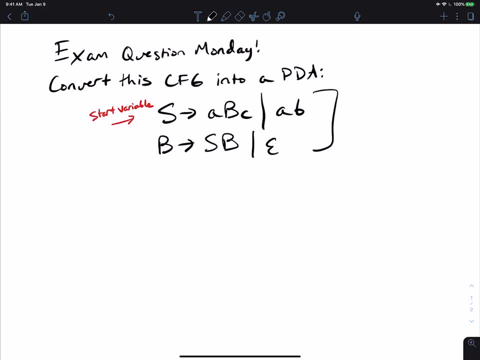 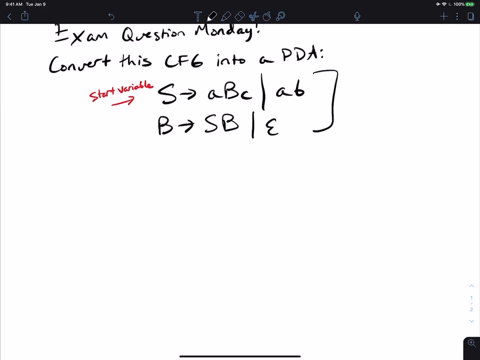 given by these two variables, s and b, and we want to convert it into a PDA. So how do we actually do that? Well, remember, a PDA has a stack and what we need to do is to utilize the stack by applying the rules on the stack. So if a terminal is on the top of the stack, we want to read it. 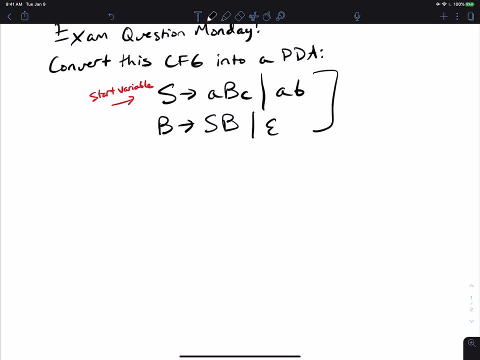 off of the input at the same time as popping it. and if there's a variable on top of the stack, then we're going to apply a rule corresponding to that variable And to make sure that the computation is correct, we're going to use a variable on top of the stack. So if a terminal 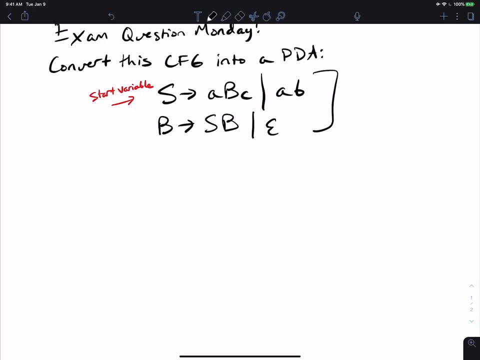 finishes correctly. we always will put a bottom-of-stack marker so that we never pop an empty stack. So what we should do then is, in the start state, we're going to not read anything. So most of these transitions will not read anything, other than ones that we'll see, a few that we'll 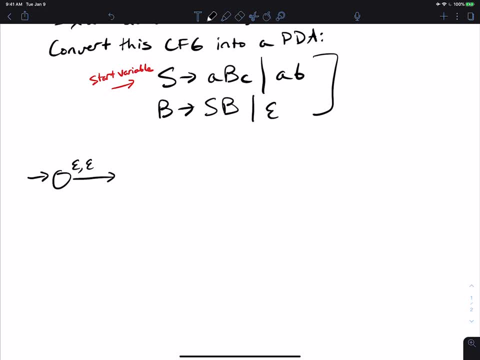 see later. So we're not going to pop anything, because we shouldn't pop when there's an empty stack. and we're going to put a dollar sign on the bottom. Well, really, any bottom-of-stack marker, a special character, is fine. So then we come to here and then 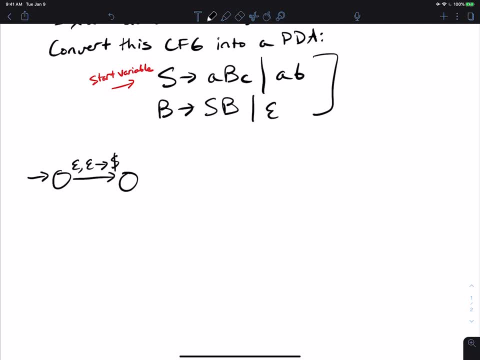 now what we're going to do is to start the derivation, because we want to simulate the derivation on the stack. Well, every derivation starts with the start variable. Well, the start variable in this grammar is s, So we're going to put s on the bottom of the stack again. 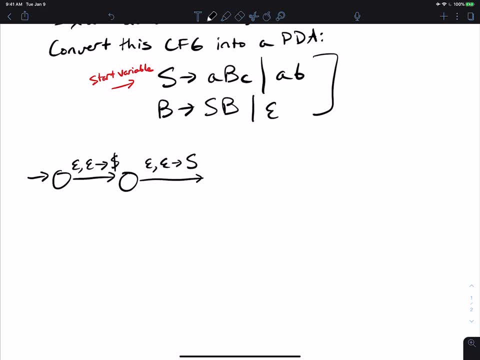 not reading anything, So and not popping anything because we want to pop the dollar sign that we just put on. So now we're going to come to a state I call QLoop, and the whole goal of this state is to assess what's at the top of the stack and decide. 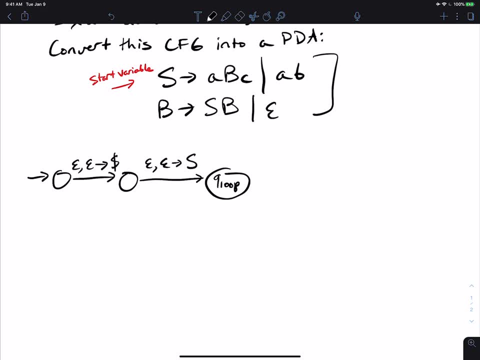 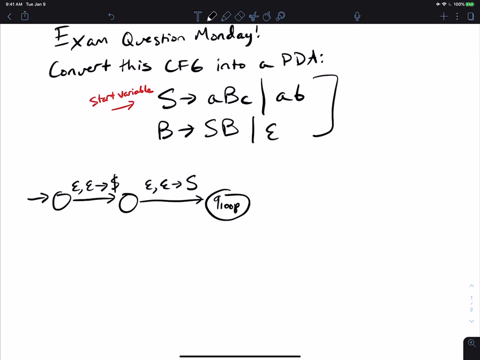 what to do from there. So if a variable's on top of the stack, then apply a rule. If a terminal's on top of the stack, read off the input at the same time as popping that character off. And if a dollar sign's on top of the stack, go to a final state, which means that you should accept at that. 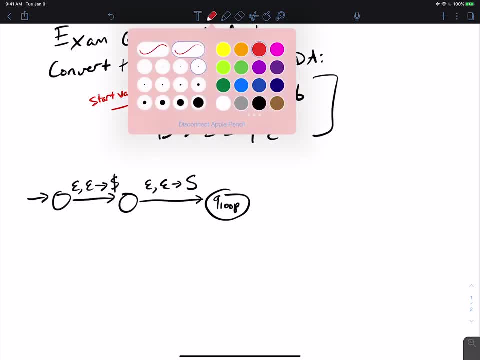 point. So let's handle the terminals. So what are the terminals in this grammar? Well, it's everything that's lowercase a, b and c. So we're going to have three self loops right here. So this will always happen for every terminal in the grammar, no matter what. So then here, 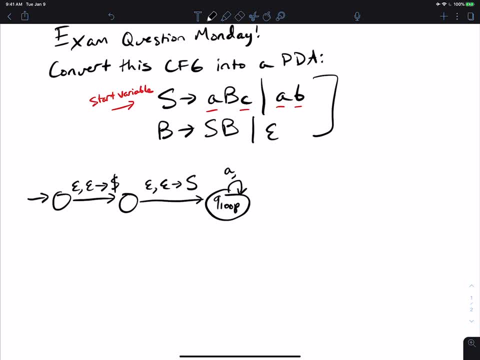 we're going to have a because we're reading off the input, always popping the same character and then pushing nothing. So, as the characters are being produced on top of the stack, they'll never change because we have a context-free grammar In the derivation. 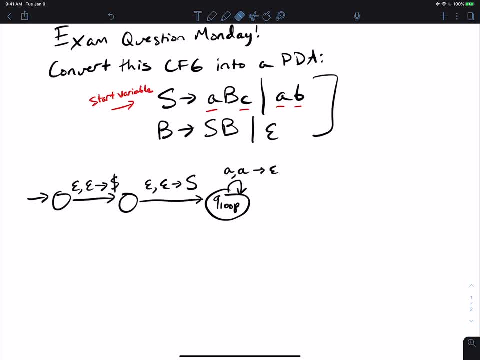 once you make a terminal, you'll never change it. So here what we're trying to do is we're trying to match off of the input at the same time that they're being produced on the stack. So then we're going to do exactly the same thing for the b terminal and the same thing for the. 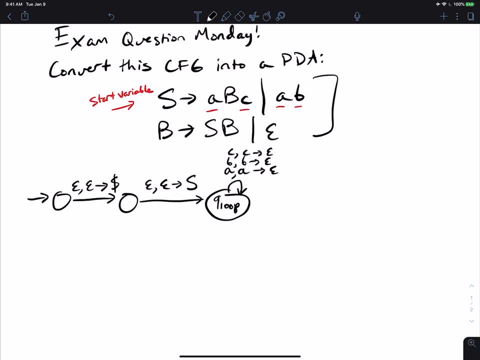 terminal. No problem, If we have a dollar sign on top of the stack, we need to go to an accept at some point. So I'm going to have epsilon dollar sign goes to epsilon go to a final state. And these four states right here, these four states, I'm going to call the base states. So 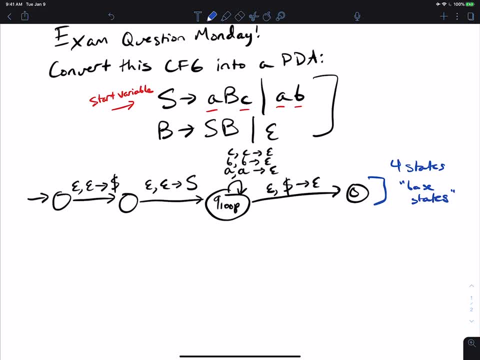 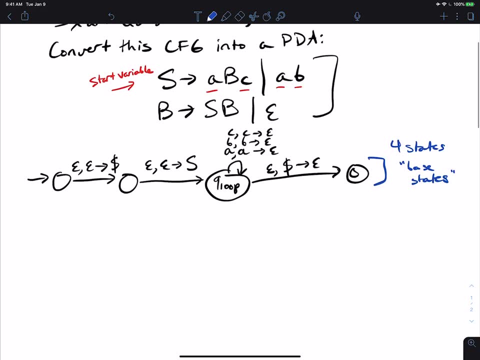 these four states will always be there. always, regardless of what the CFG looks like, It'll always be there. But now we need to handle the rules. So what we need to do is to make a series of transitions that go out from QLoop and then eventually come back to QLoop, And what we're doing is we're 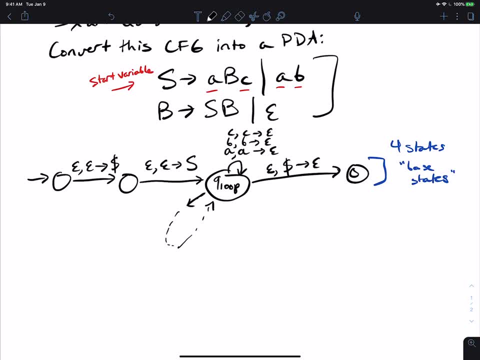 going to pop a variable off the stack and then push on the right-hand side of one of its rules. So, for example, if we are doing the rule S goes to A, B, C, then if an S is at the top of the stack. 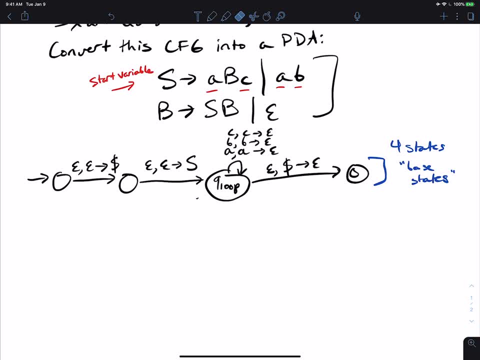 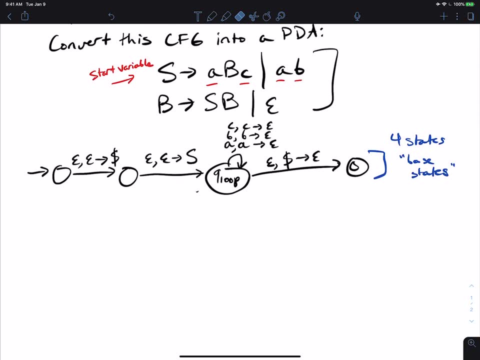 then, eventually, when we come back to QLoop, we want to have A, B, C on top of the stack. So where A, the terminal in this case is at the top, which means that we need to push on the right-hand side of the rule. 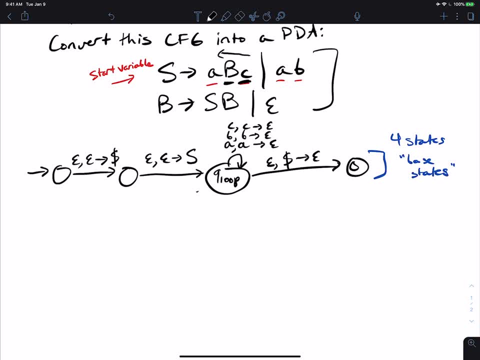 first. We need to push the C on first, then the B, then the A, because of how a stack works, A stack needs to have its last thing on the top And we want the A on the top, so we want to push it last. So let's handle S goes to A, B, C. How we're going to do that. 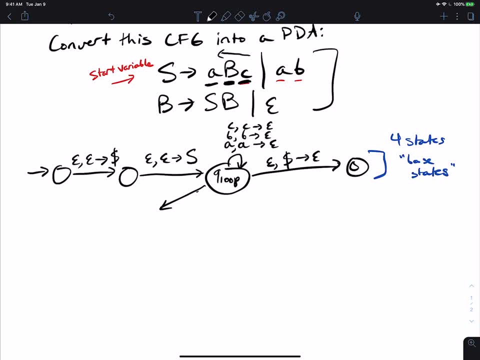 well, what we're going to do is we're again not going to read anything, So the only transitions that read are these ones right here. So maybe we'll mark this here. So these are the only transitions that read, Because in all, 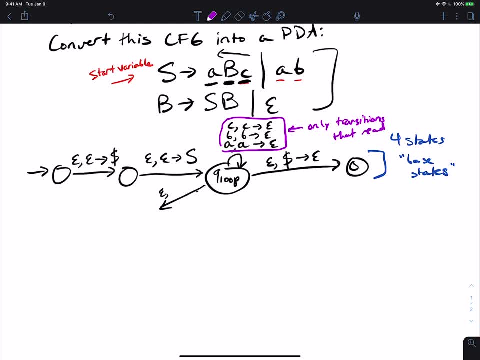 of the cases, we're going to be applying a rule, and the only time that we're going to be consuming characters is when a terminal is produced, which means that they're at the top of the stack, which means these are the only ones that are going to read anything. So this one doesn't read. Here we got. 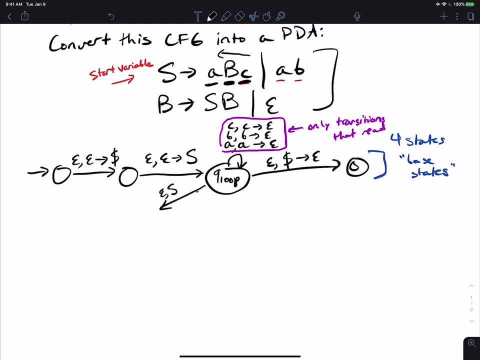 to be able to pop an S off in order to be able to apply this rule. And what I'm going to do here to save space is I'm going to push the C on immediately, because we have to push the C on first. Then we need to push on the next thing after the C- actually, I guess, before the C. 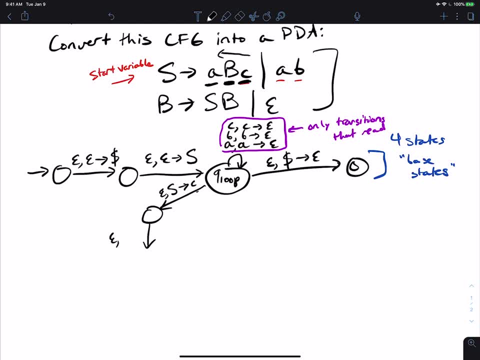 which is the B in this case. So what we're going to do here is we're going to do the same thing on the left side, So we're going to do this for every one of the cells in the grammar. So we'll do this. let's say: epsilon, epsilon. 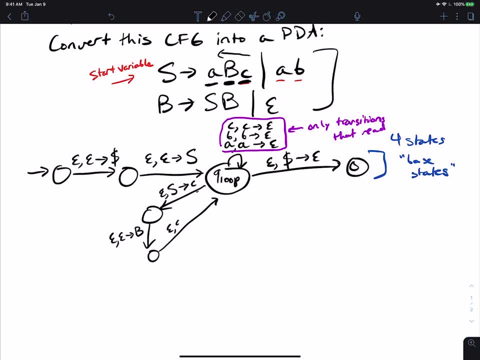 because we're not popping. anything goes to B, And then we'll come back with the last thing, which happens to be an A in this case. So epsilon, epsilon goes to A, And we'll do this exact same procedure for every rule in the grammar. So let's do so. we did S goes to A, B, C. Now let's do S. 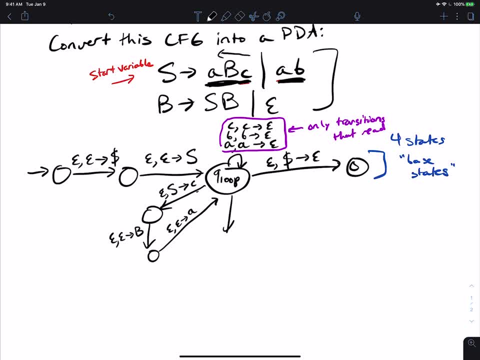 goes to A little, a little b So is have another set of transitions that go out and come back. so epsilon s goes to b, because we have to push the b on first, since it's last, and then we got to push the a on first. that i mean next. 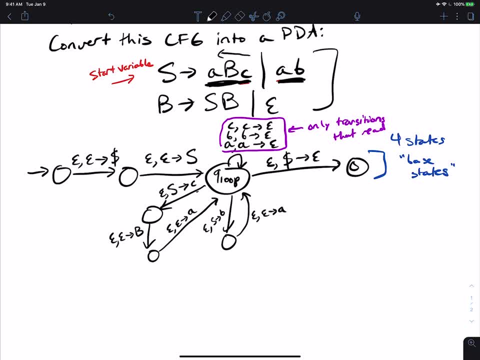 and go back to q loop. for that reason, two more to go. let's do s. sorry, b goes to sb. so then here i'm gonna have again epsilon. no read: we gotta pop off the variable on the left side of the rule, which is b in this case, and then we're going to push on the, the rightmost thing in the rule, which 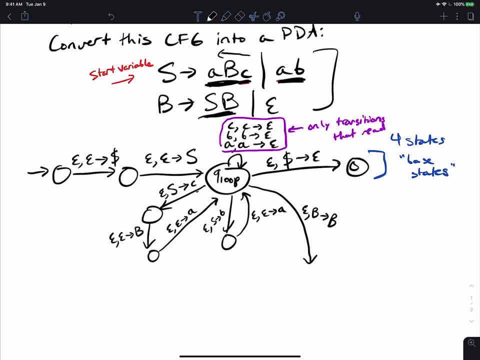 happens to be b. so, effectively, this rule does nothing, except we can only take it if the b appears at the top of the stack. so then we come to a state and let me squeeze this in here. so this will be epsilon. epsilon goes to s, and then, finally, i'm going to squeeze in a self loop. 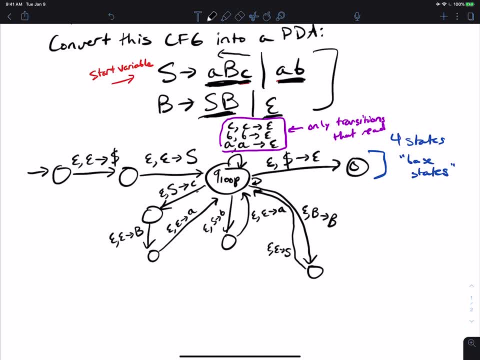 right here, because for the epsilon rule we can just do it in one transition instead of two. so here we're going to have epsilon b, because again, we want to apply this rule and we can only do it if the thing that is on the top of the stack is a, b, and we don't want to push anything because 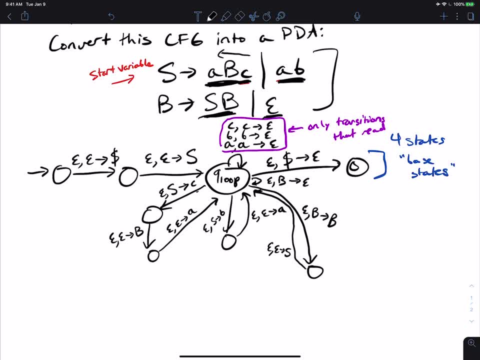 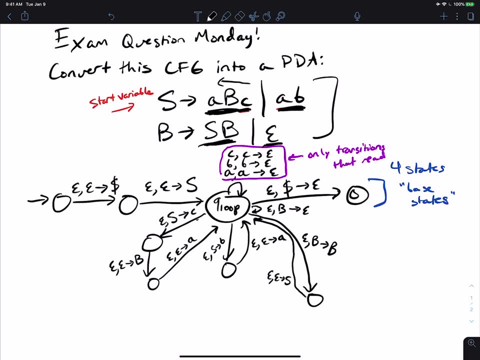 there's. there's nothing on the right side of the stack, so we're going to do that and we're going to do that on the right hand side, and there we go. so the thing to take home from this is the four base states are always going to be the same. you're always going to push on the start, a special 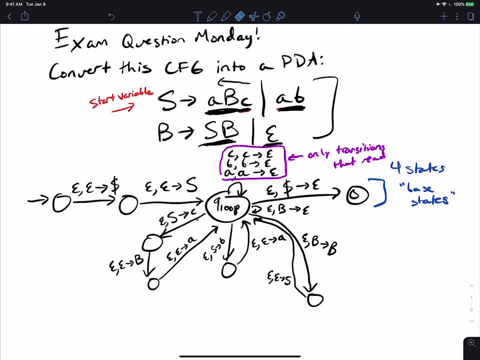 character, then the start variable go to a state called q loop, and then you're going to have epsilon. the special symbol goes to epsilon, to a final state. the q loop state always has self loops on every turn, and so you can do those for all of the functions that are in the cfg. and the first thing that we